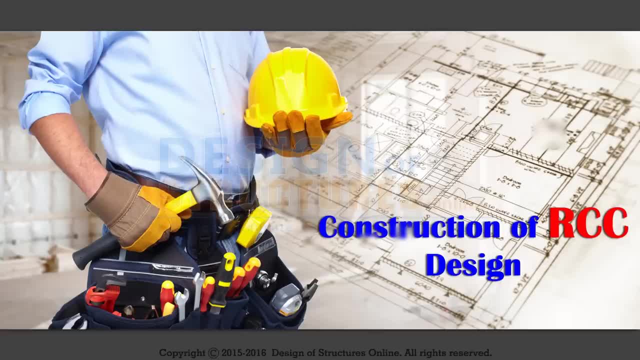 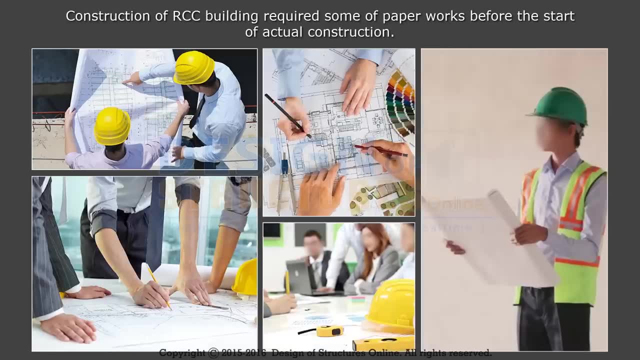 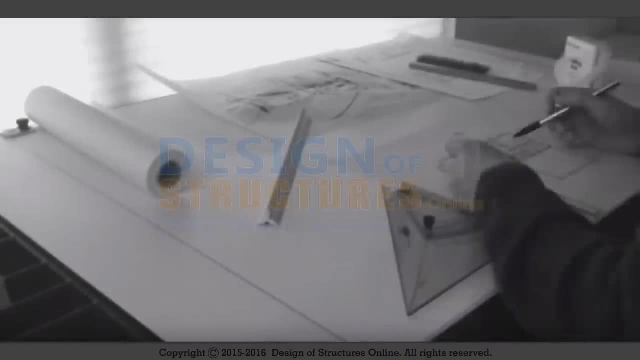 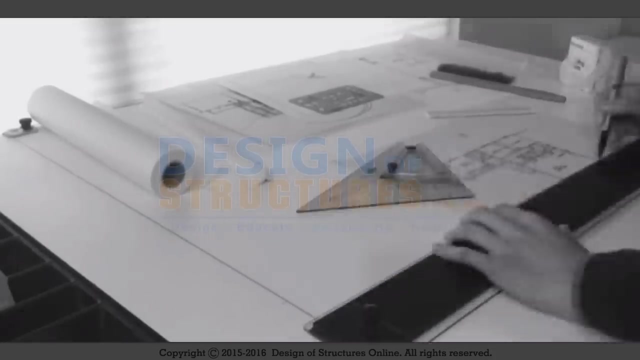 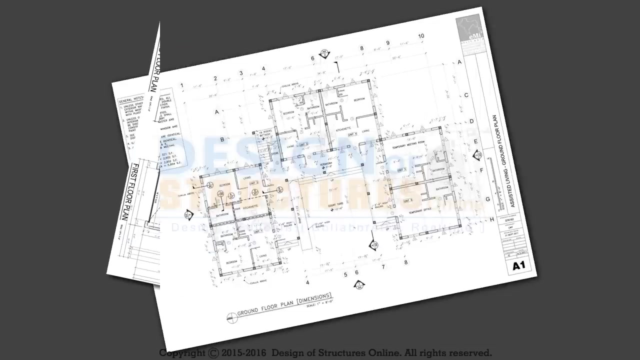 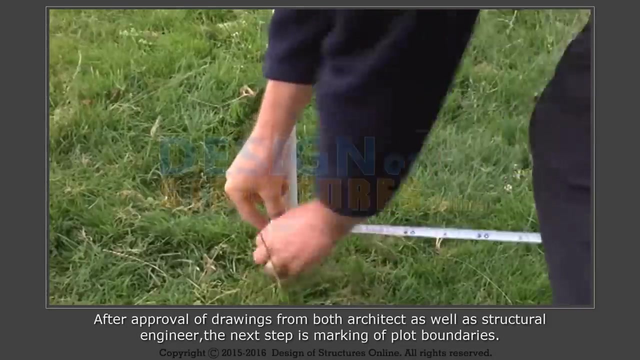 Construction of RCC design. Construction of RCC building required some of paper work before the start of actual construction. The very first stage is preparation of drawings as per requirements of client. Once drawings are completed, approval of drawings is important. After approval of drawings from both architect as well as structural engineer, the next step is marking of plot boundaries. 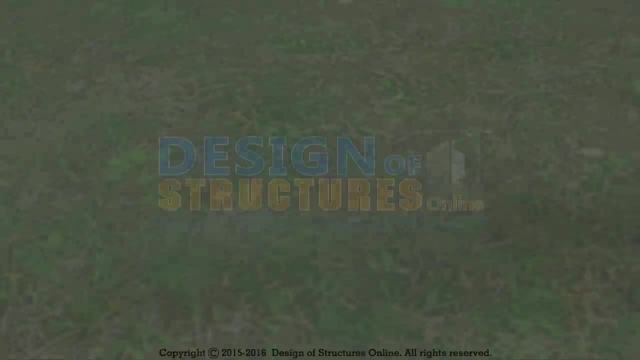 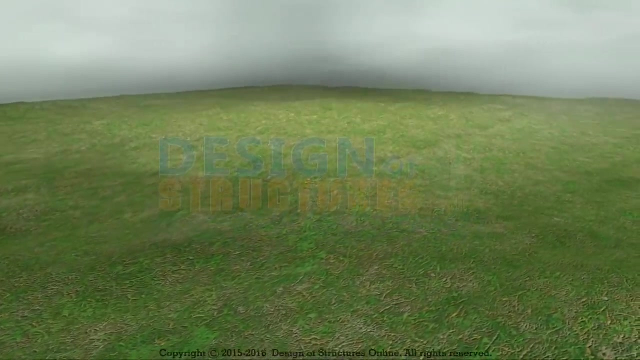 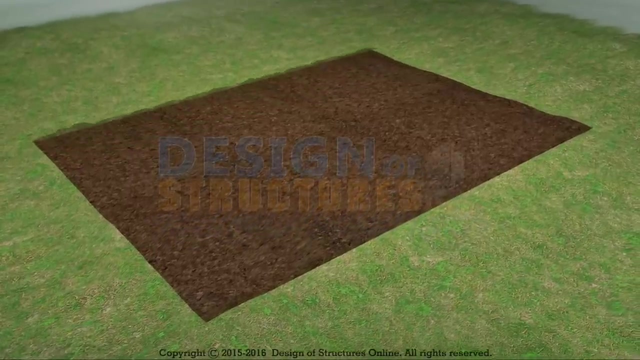 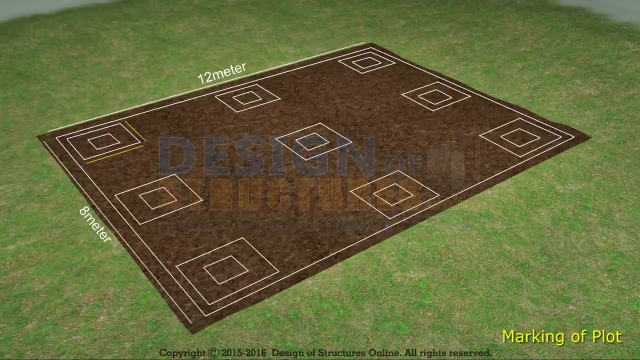 Cleaning of plot. Site preparation consists of clearing away the trees from your building site. This involves the removal of trees, roots and other vegetation from the building site. After cleaning the site plot, marking of plot should be done as per drawings. Excavation- 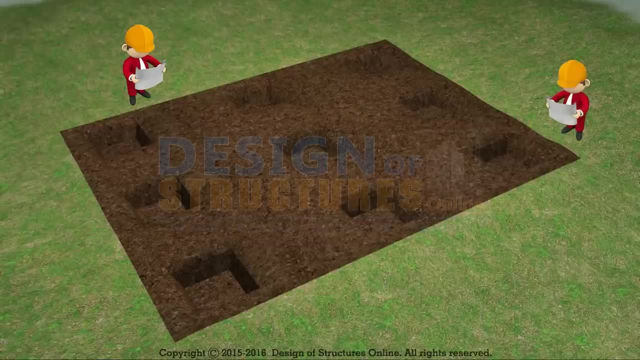 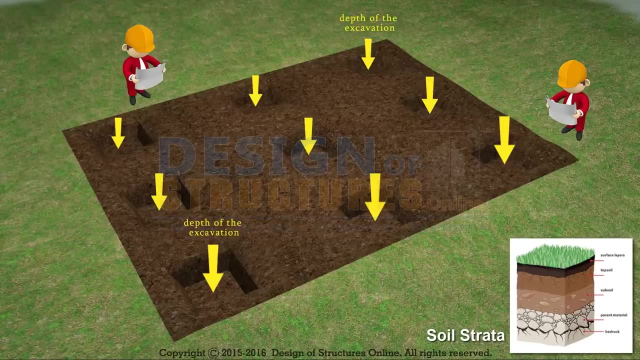 A structural engineer will be needed to determine the depth of the excavation. The depth will vary as per building, depending upon soil strata. Excavation should be carried out as per the drawings defined lengths and widths. Excavation is to be done by the JCB. 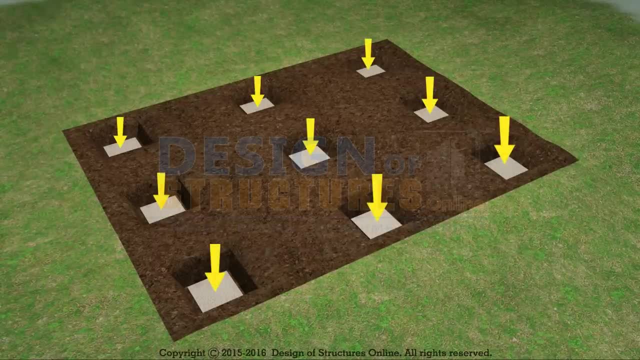 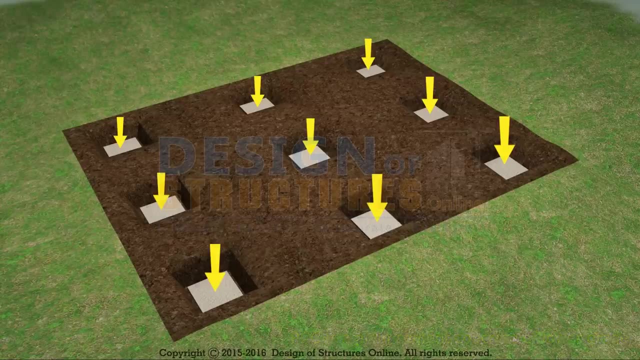 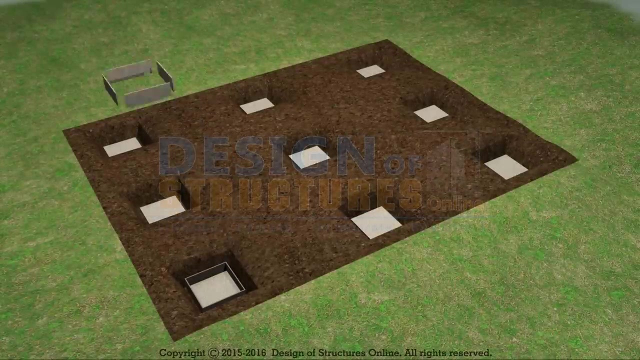 PCC. After the excavation: the surface is leveled. PCC poured over leveled surface. Excavation is to be done as per the drawings, defined lengths and widths. Foundation shuttering: Shuttering: arrangement for foundation is to be made Once PCC is done. shuttering for foundation is placed. 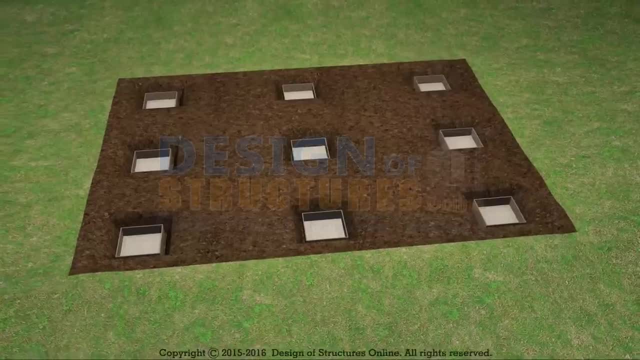 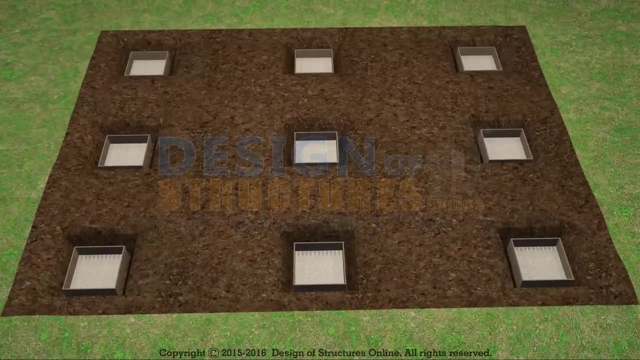 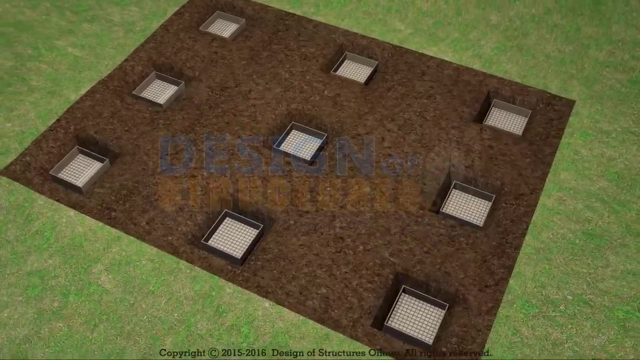 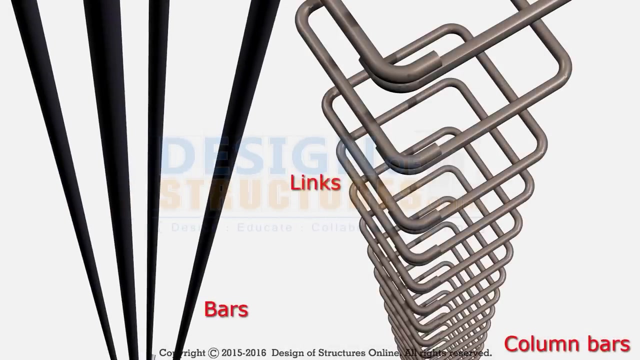 It should be strong enough to withstand all types of dead and live loads. Foundation bars: Foundation bars shall be laid on the surface. Main bars and distribution bars shall place as per drawing. Column bars: Column bars: Proper arrangement to be made for column bars with links as per drawings. 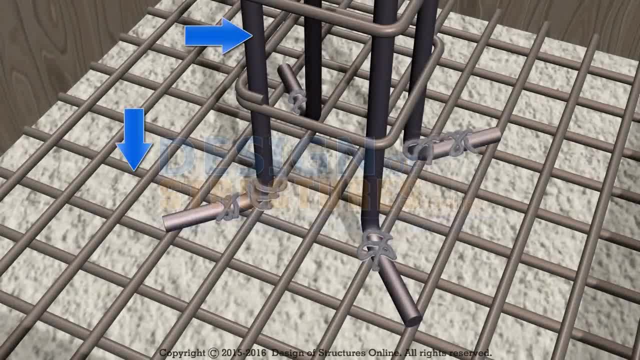 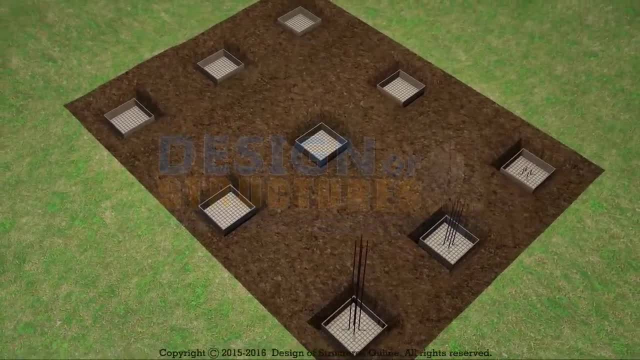 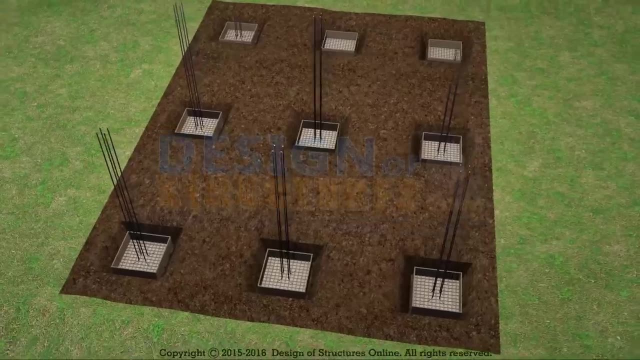 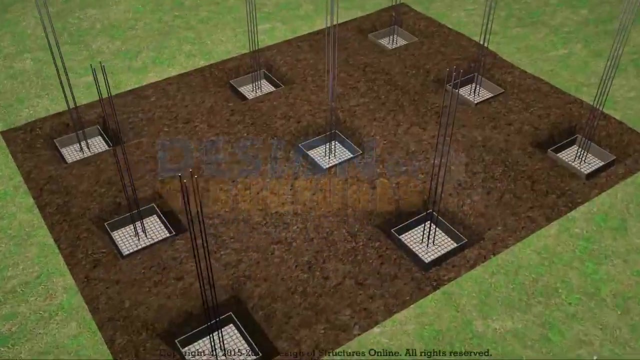 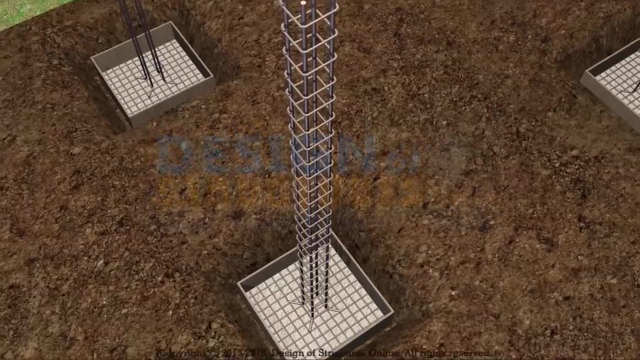 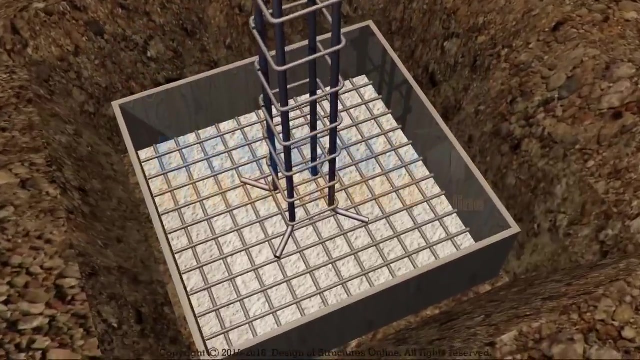 Column steel and foundation steel to be tied properly to avoid joint cracks. Reinforcement shall be as per bar bending schedule prepared according to drawing. The reinforcement shifting and binding shall be started as soon as shuttering is completed. Reinforcement binding shall continue as shuttering work as progresses. 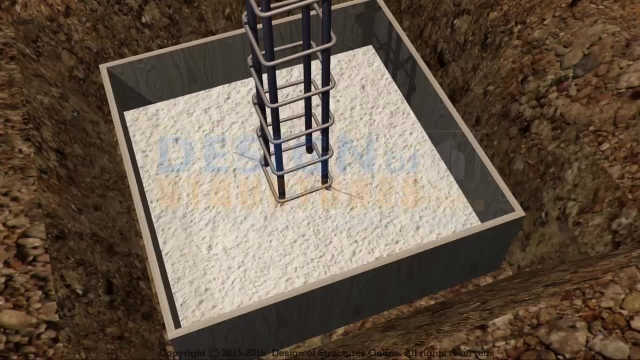 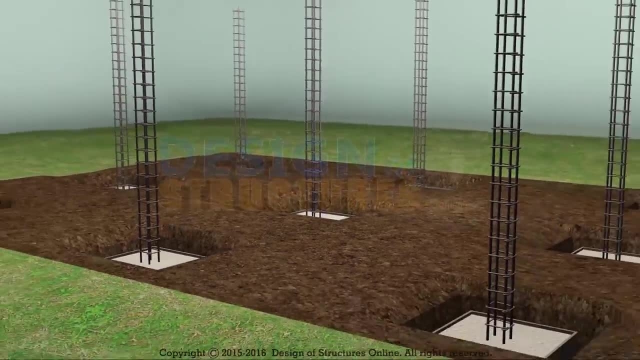 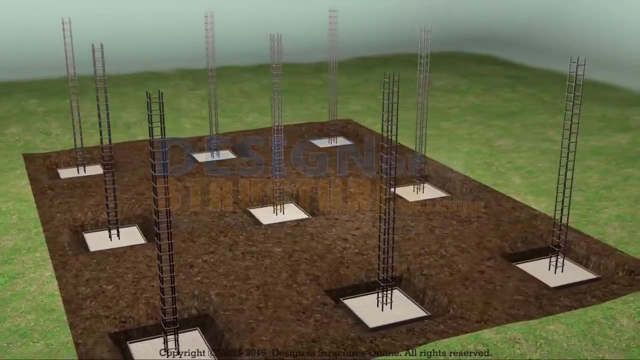 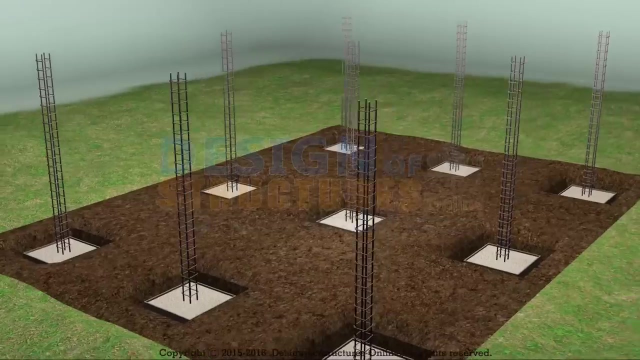 Concrete work in foundation. Concrete work in foundation. A foundation is a poured concrete pathway that is used to spread the weight of the building from bottom to top. The foundation is used to adjust the weight of the building from the foundation to the soil. It is very necessary to check the levels of foundation before concrete work. 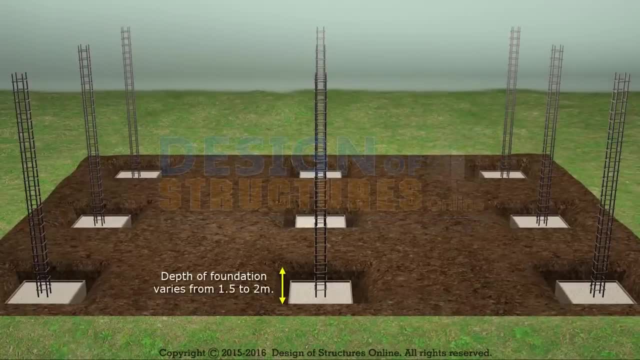 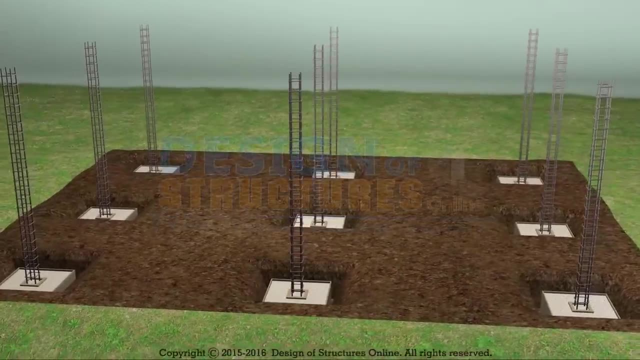 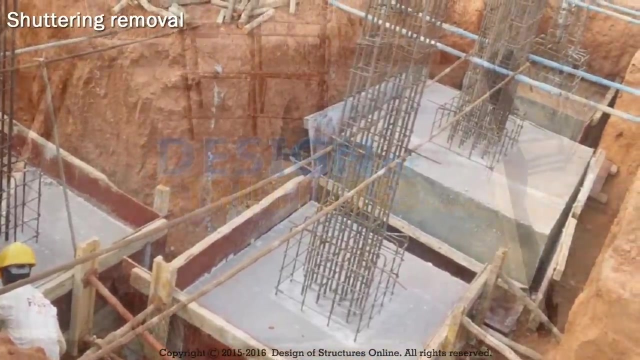 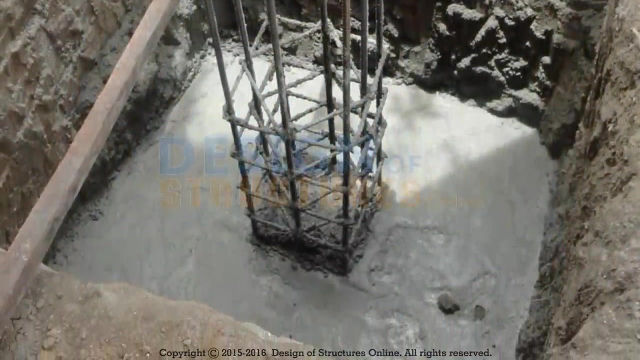 Bottom level Cu 1938 Shattering Removal. The formwork removal procedure should be supervised by the engineer to ensure that quality of hardened concrete in structural member, That is, it should be free from or has minimum casting defects, such as honeycombing, size and shape defects, etc. 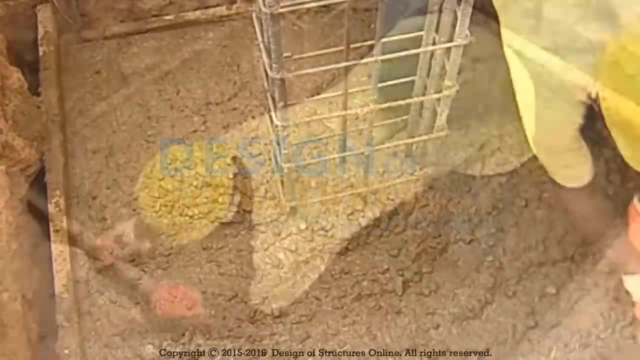 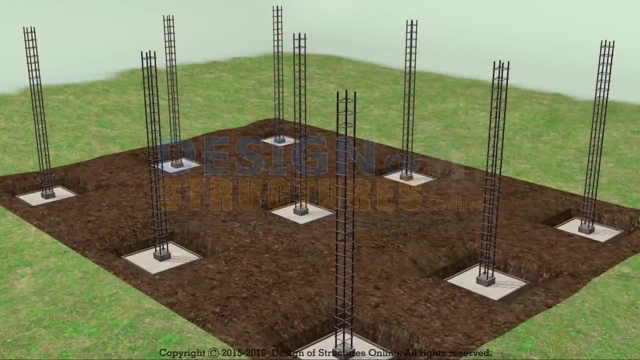 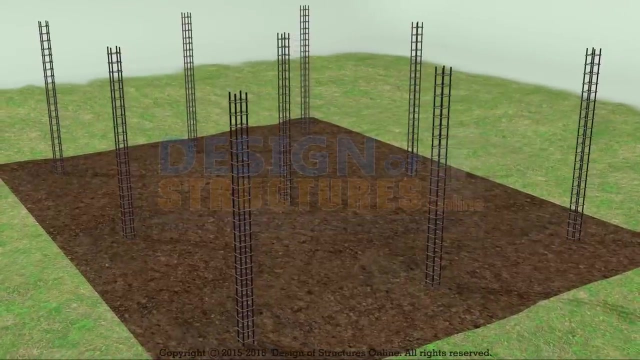 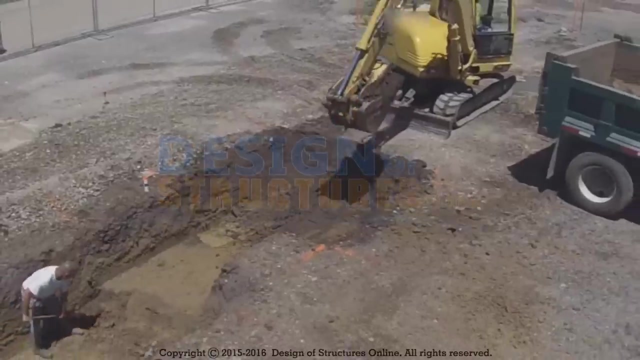 These defects in concrete influence the strength and stability of structure. thus, immediate repair works can be done or the members can be rejected. Backfilling Once the foundation is completed: backfill the remaining excavated area around foundation with soil. Backfill provides stability to the building. a Euro trademark S foundation. 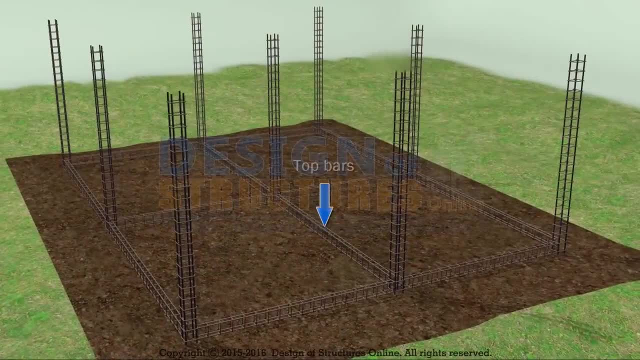 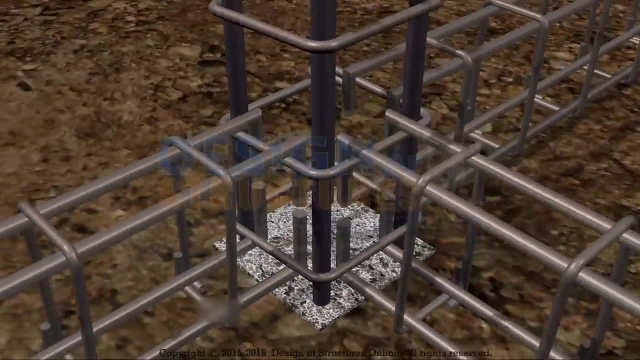 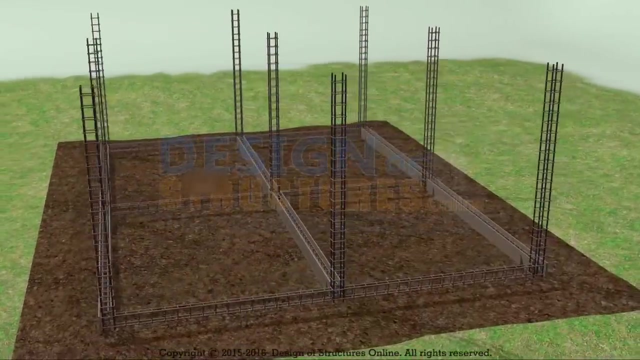 Beam reinforcement. Beam reinforcement shall be as per drawings: Top bars, bottom bars and stirrups to be placed with proper development length. Joints in the beam shuttering should be tight against leakage of cement grout. Construction of shuttering should permit removal of various parts in desired sequences without damage to the concrete. 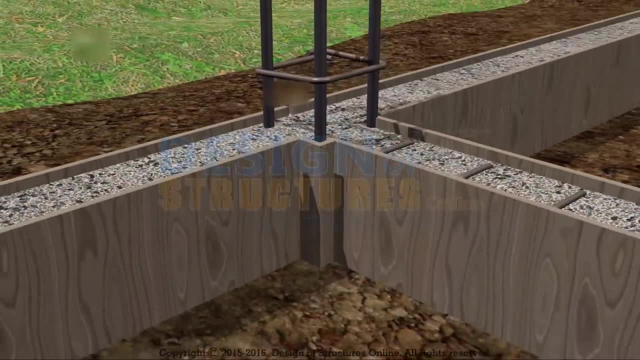 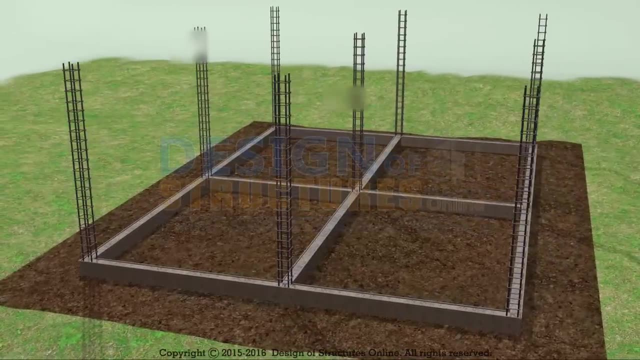 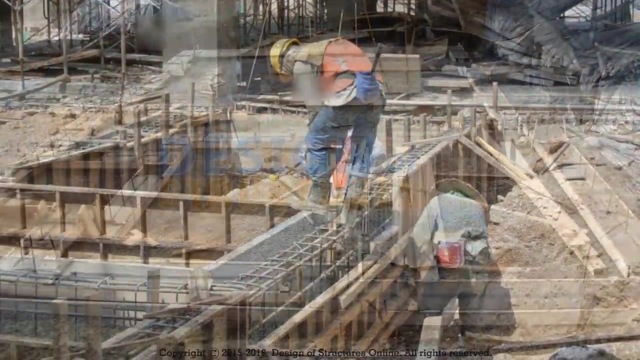 Beam- concreting Beam. concreting Beam is poured with concrete, Concrete with grade mentioned in the drawings. The positioning of reinforcement should be properly aligned. Shuttering parts and connections should be arranged in a way that makes formwork removal easy and simple, prevents damage to concrete and formwork panels so that it can be reused without extensive repair. 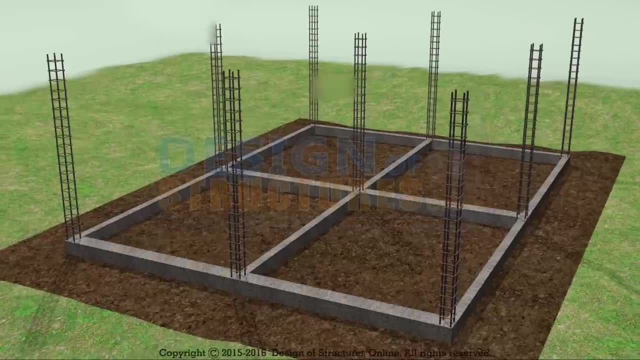